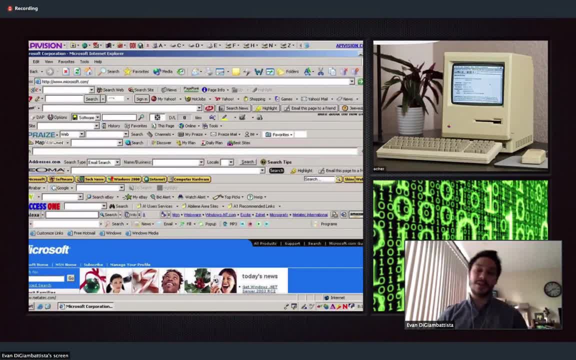 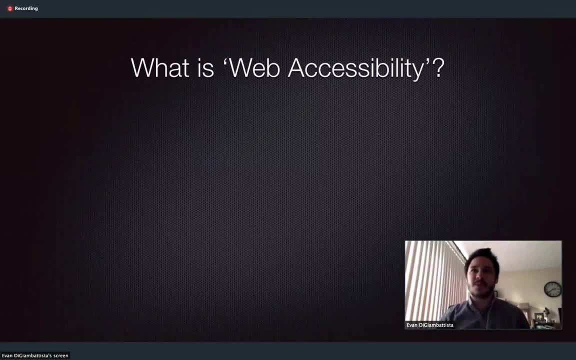 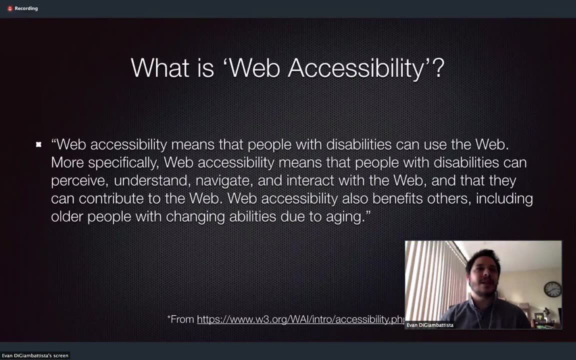 across all types of platform and for all types of user. And that's just a screenshot of my computer Desktop. it's okay. So what is web accessibility? Well, according to the W3.org website, web accessibility means that people with disabilities can use the web. More specifically, web accessibility- 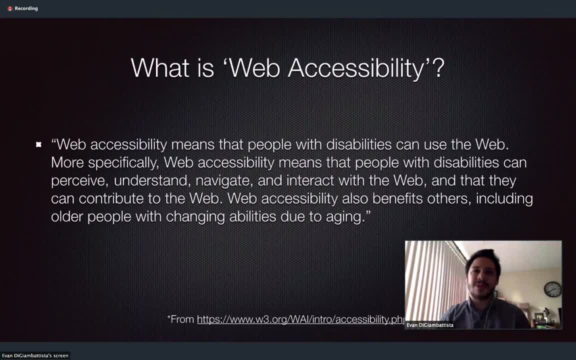 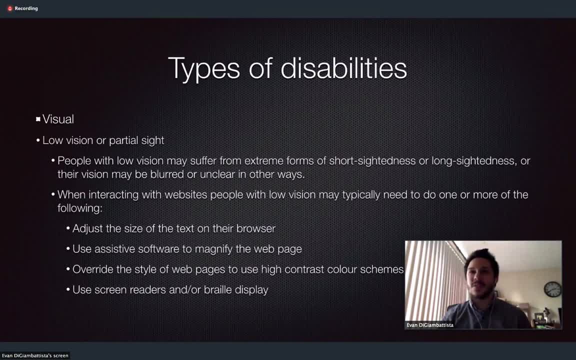 change your life. If you're a person with a disability, you can use the web to change your life. If you're a person with a disability, you can use the web to change your life If may typically need to do one or more of the following: 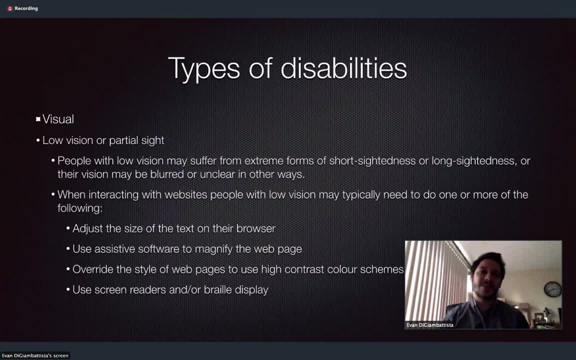 They may need to adjust the size of text on their browser. They can also use assistive software to magnify the webpage, override the style of webpages, to use high contrast color schemes or use screen readers and or braille displays. And that's from coolfieldscouk, which was a cool site. 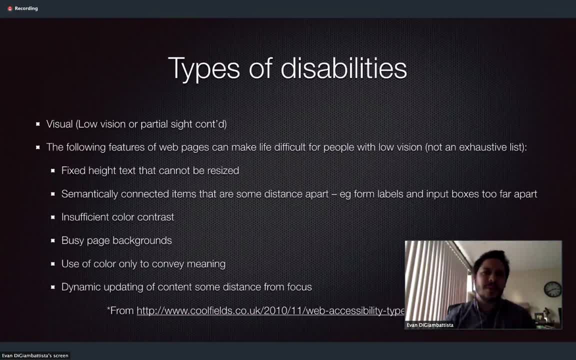 So low vision or partial sight continued. These things sort of make life difficult for people with low vision or partial sight. Fixed height text that cannot be resized semantically connected items that are some distance apart, ie form labels and input boxes, are too far apart. 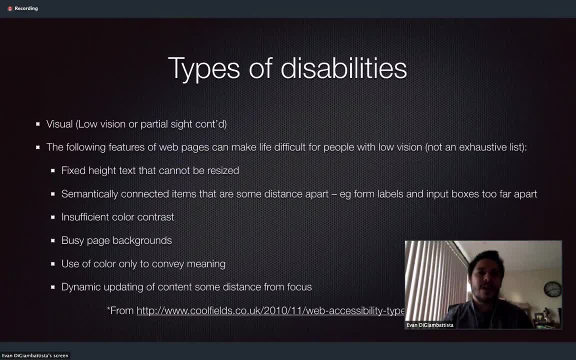 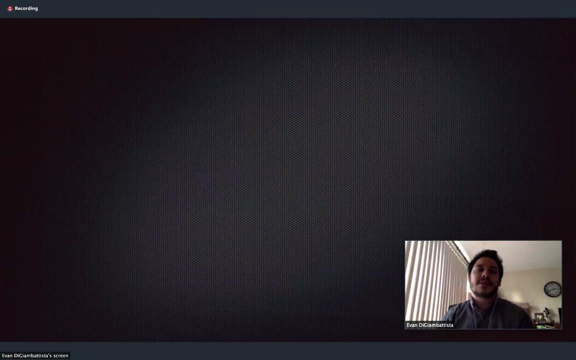 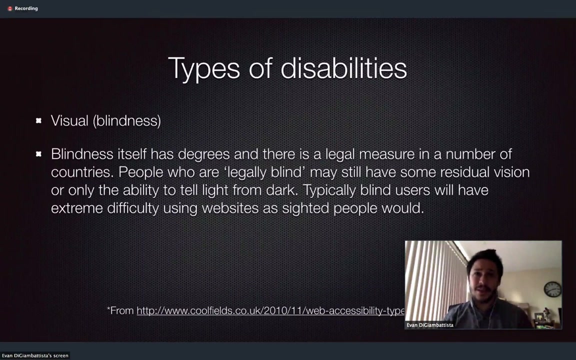 color contrast, busy page backgrounds, using color to only convey meaning, and dynamic updating of content from some distance from focus. Yeah, So we also have blindness. Blindness itself has disagrees that and there is a legal measure in a number of countries. 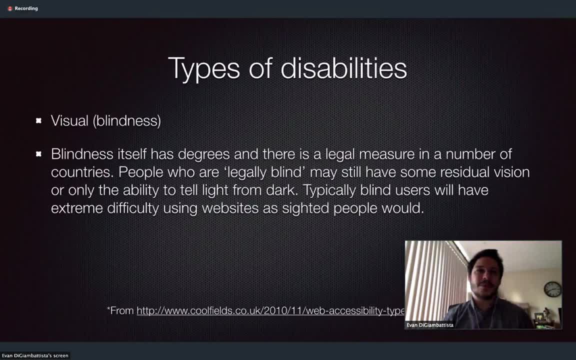 people who are legally blind may still have some residual vision. or- and there is a legal measure in a number of countries- people who are legally blind may still have some residual vision or only the ability to tell light from dark. Typically blind users will have extreme difficulty. 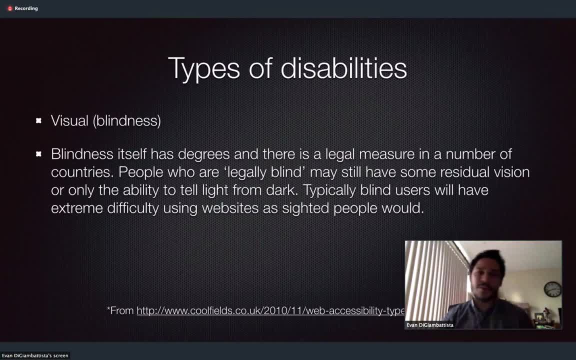 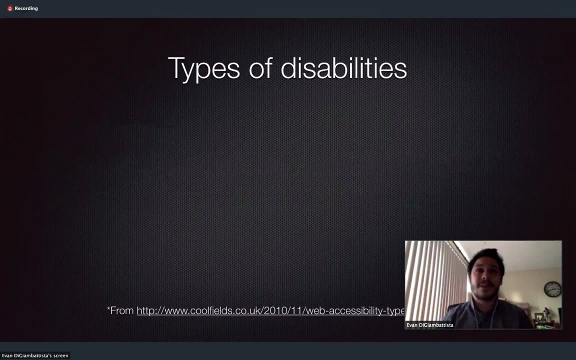 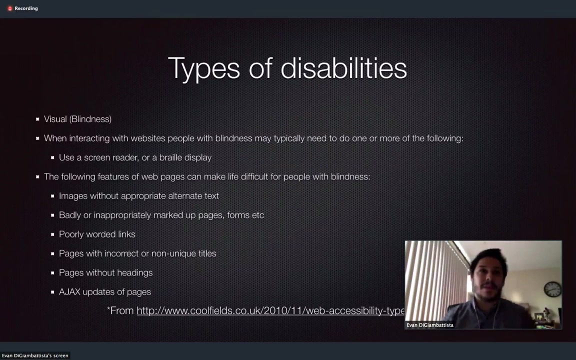 using websites, as sighted people would, And this is sort of where screen readers kind of come into play. If you can imagine not being able to use your mouse or your eyes at all, how would you manipulate anything on the computer? Okay, So, like I said before, 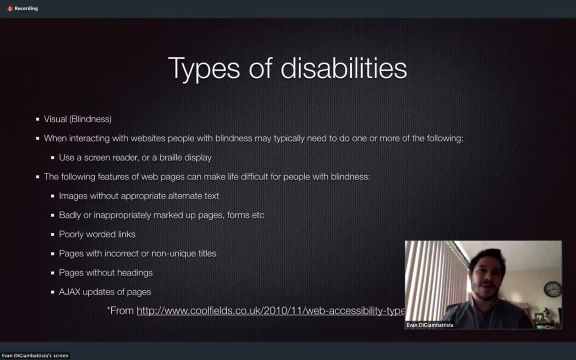 people who are blind will use a screen reader, Braille display and these are some things that sort of make life difficult. Images without appropriate alternate text: that would be sort of like the alt attribute on an HTML tag: badly or inappropriately marked up pages or forms. 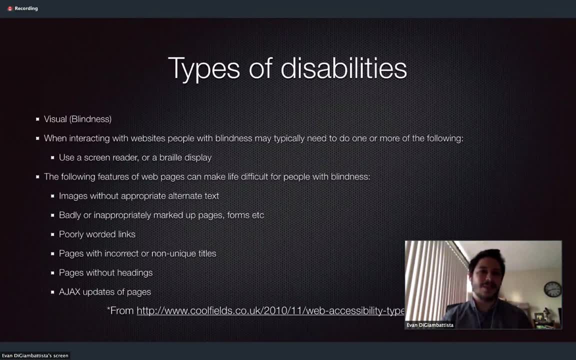 poorly worded links. pages with incorrect or non-unique types titles. pages without headings- Headings are actually really important, just to allow a user to know exactly where and of what important things on a page are- And finally, Ajax updates. 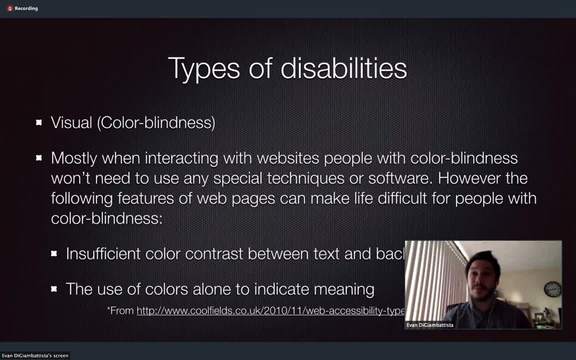 So there's also colorblindness. Mostly when interacting with websites, people with colorblindness will need to use any special techniques. However, the following features can make life difficult: Insufficient color contrast between text and background and the use of colors alone to indicate meeting. 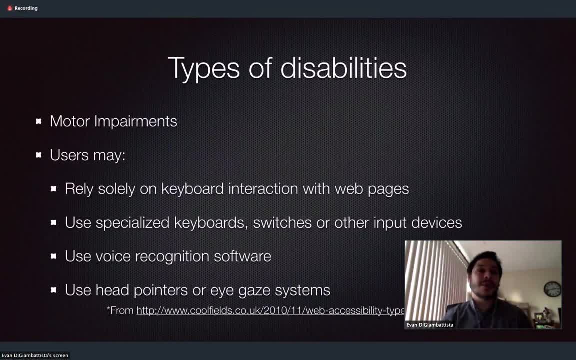 Whoops. Motor impairments. Users will rely solely on a keyboard interaction with web pages. They may use specialized keyboard switches or other input devices. They may use voice recognition. They may use voice recognition software And they may use head pointers or eye gaze systems. 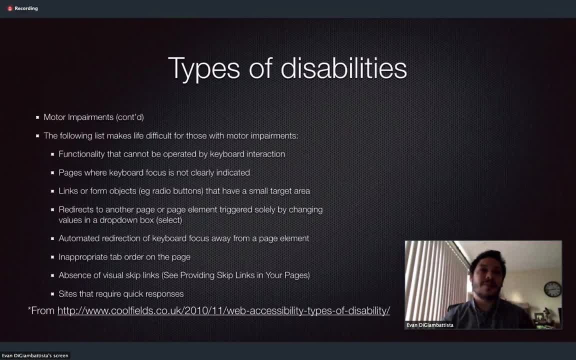 Motor impairments continue. These things make life difficult. Functionality that cannot be operated by keyboard interaction. Pages where keyboard focus is not clearly indicated. Links or form objects. radio buttons that have a small target area. redirects to another page or element triggered solely by changing values. 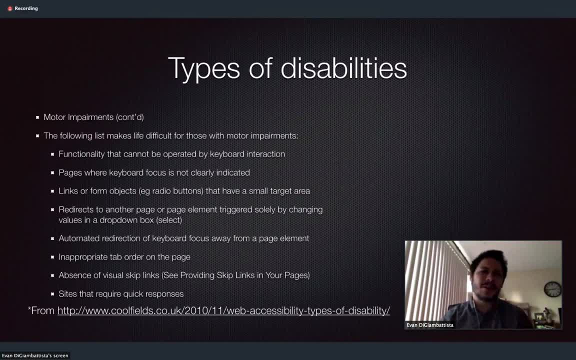 in a drop-down box like a select. Automatic redirects of keyboard focus away from a page element. Inappropriate tab order on the page. Absence of visual skip links: See providing skip links in your pages. Actually, I don't know what that is. 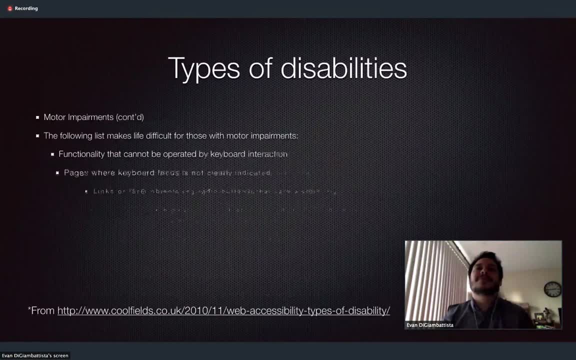 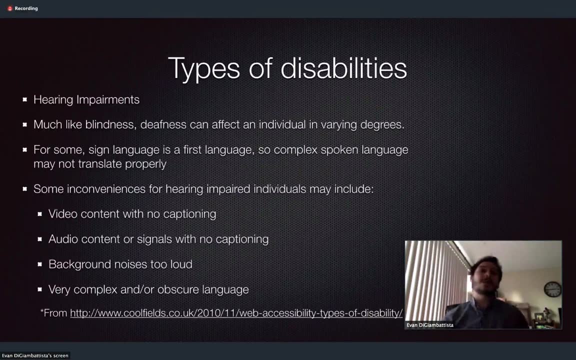 Sites that require quick responses, Moving right along. Hearing impairments. Much like blindness, deafness can affect an individual in varying degrees. For some, sign language is a first language, So complex spoken language may not translate properly. Some inconveniences for hearing impaired: 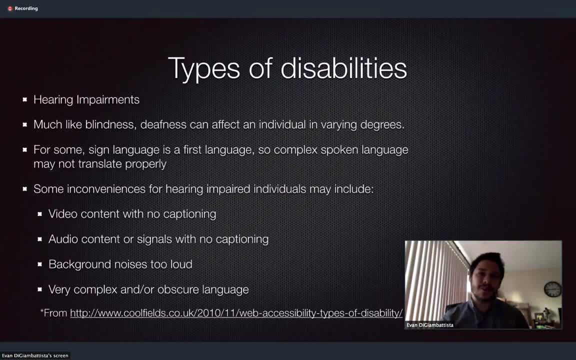 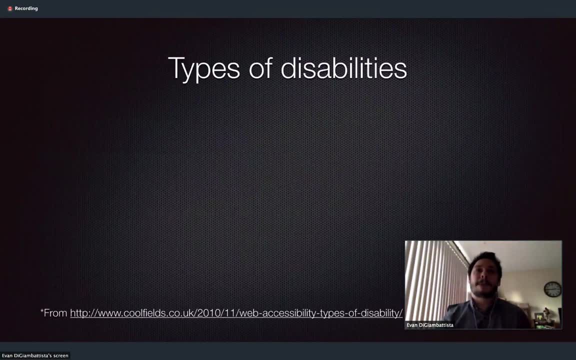 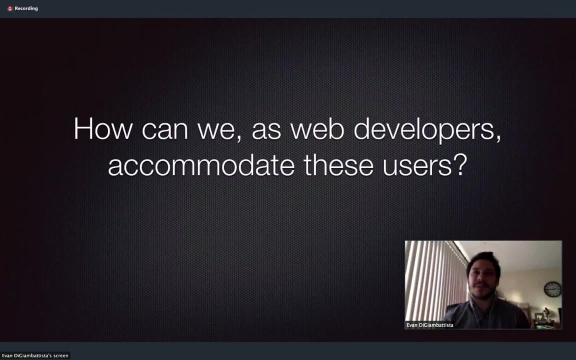 would be video content with no captioning, audio content or signals with no captioning. background noise is too loud or very complex, and or obscure language, All right. so how can we, as web developers, accommodate these users? There's something called ARIA. 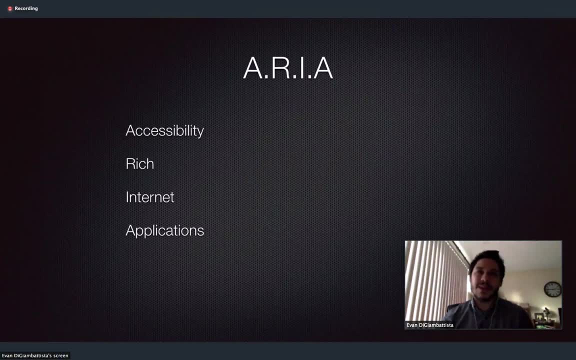 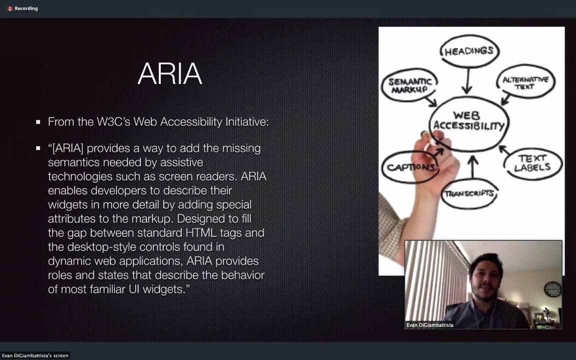 And ARIA stands for Accessibility, Rich Internet Applications And from the W3C website. ARIA provides a way to add the missing semantics needed by assistive technologies such as screen readers. ARIA enables developers to describe their widgets in more detail by adding special attributes to the markup. 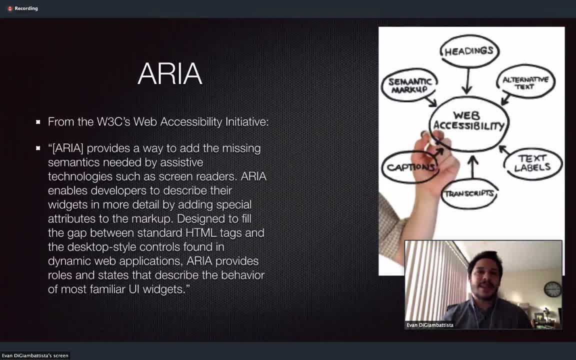 Designed to fill the gap between standard HTML tags and the desk top style controls found in dynamic web applications. ARIA provides roles and states that describe the behavior of most familiar UI widgets, And this picture here, I think, is a really good explanation of sort of what we can do as web developers. 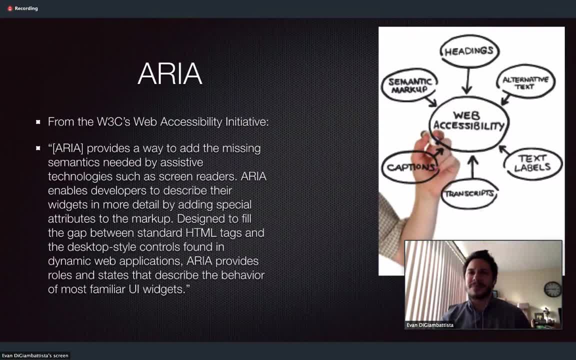 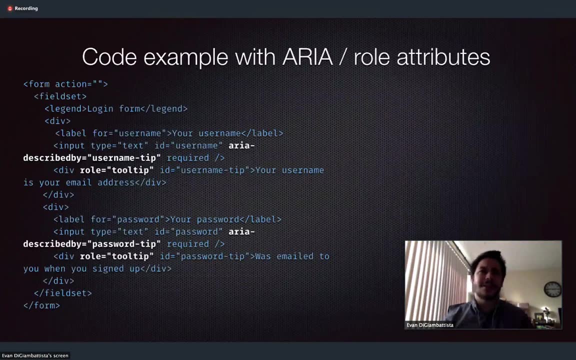 to start creating more descriptive tags, headings, alternate text, text, labels, transcripts, captions, semantic markups, all these things kind of play together to And provide a more accessible experience. So finally, some code examples. This one is of a form. 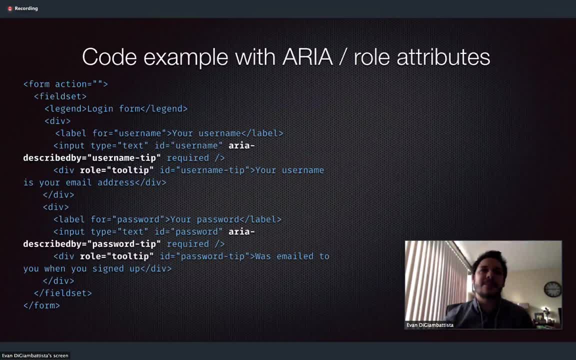 And under the field set we have a div that has a label for username And then under that the input has the ID of username And then we have an ARIA described by username tip. So under that is a div with a role of tool tip. 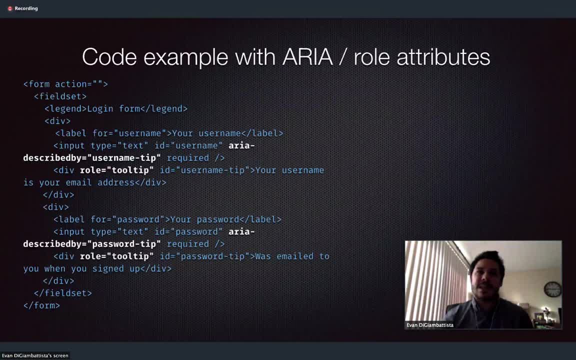 So, and then the ID matches the ARIA described by tag, And we'll actually see this later. I have a working demo of this. It's just a tool tip on a form, But it describes to the user that there is a tool tip that will happen. 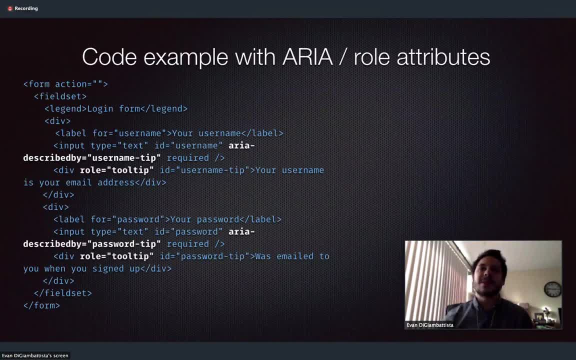 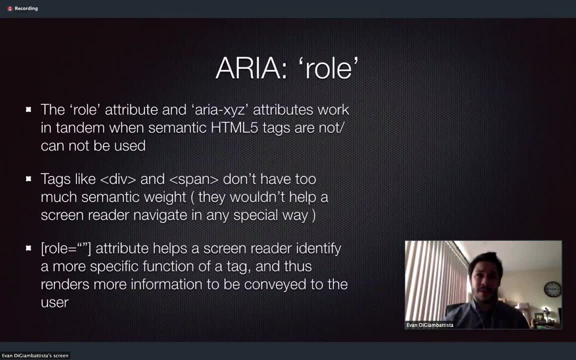 And it conveys some information in case you need more information. And then on the bottom is sort of the same thing for the password field. The role attribute works kind of in tandem when semantic HTML5 tags cannot be used, So tags like div and span they don't really. 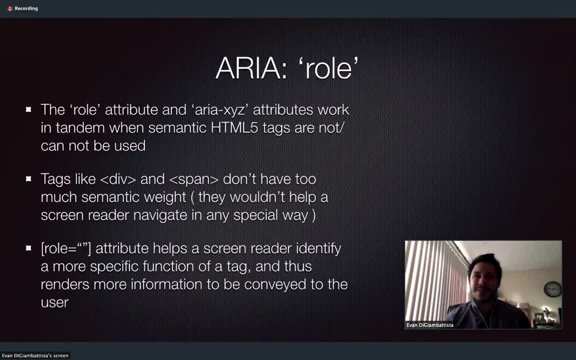 describe too much about what is happening on the page, So screen readers really wouldn't have an easy time knowing what's going on with a div or a span. So the role attribute helps the screen reader identify more specific function of a tag and thus renders more information. 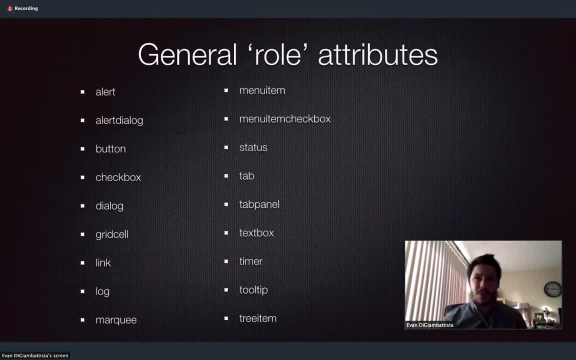 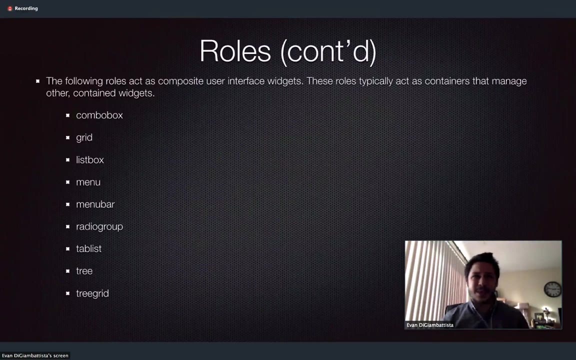 to be conveyed to the user. Here are some general role attributes. Imagine having a span or a div, And if you have a role of marquee, then that's more descriptive to a screen reader. Then these ones act as composite user interface widgets. 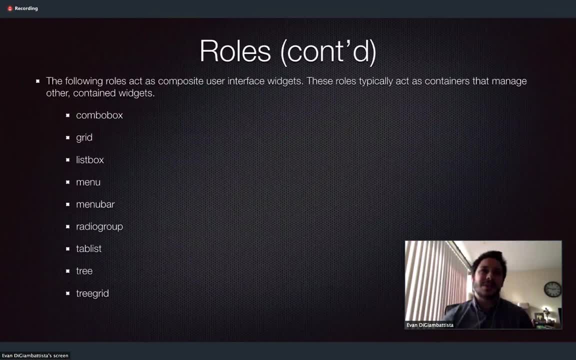 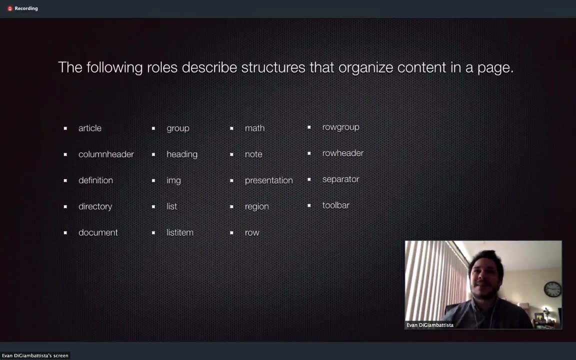 So they are sort of like containers for other widgets, So a menu or a tree tabless menu bar get the picture Structures that organize content in the page. So these are kind of grander, So article stuff, like toolbar it's. 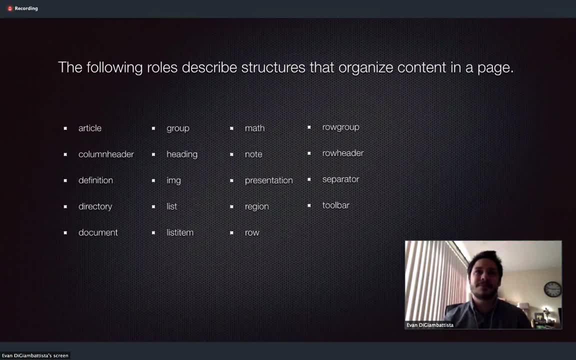 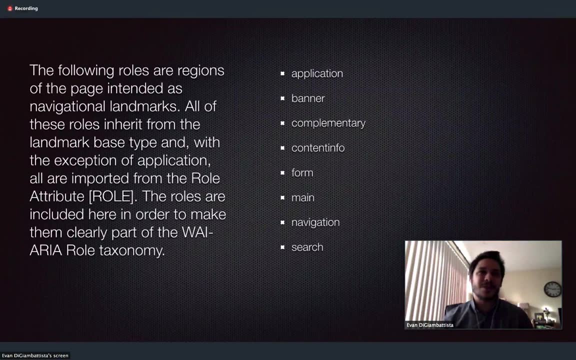 a little bit more general, holds other widgets And the following roles are regions of the page intended as navigational landmarks. All these roles inherit from the landmark base type And, with the exception of application, are imported from the role attribute. So you can see some of these are actually. 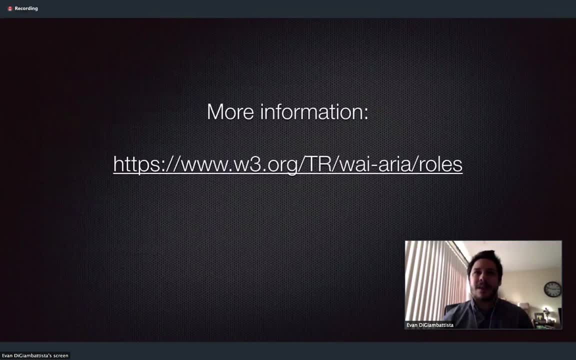 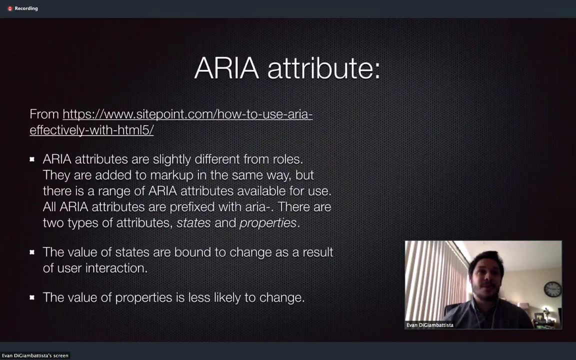 included in the HTML5 semantics. Obviously, more information can be found at w3.org. And the attribute so from SitePoint. SitePoint was actually a really good resource. Basically, ARIA attributes are slightly different from roles. They are added to markup. 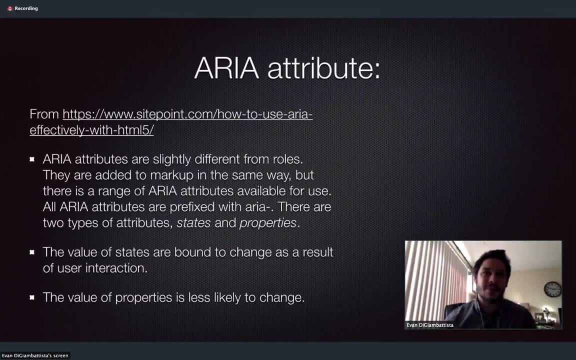 And you can see that there are a number of ARIA attributes that are added to markup in the same way, But there is a range of ARIA attributes available for use. All ARIA attributes are prefixed with ARIA dash something. There are two types of ARIA attributes, pretty much state. 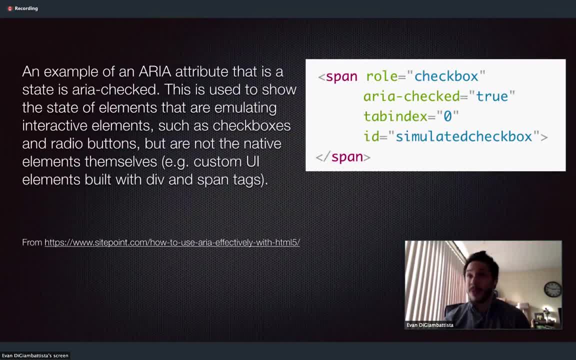 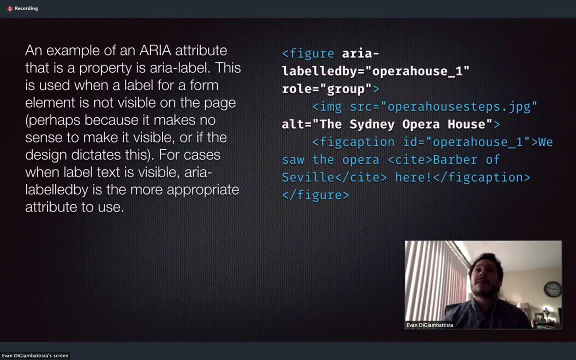 and property. So, as you can see, to the right, here we have a span, not descriptive, But we have a role of checkbox and an ARIA checked which is describing some state of true. So let's see, So we have a property, that is a property is ARIA label. 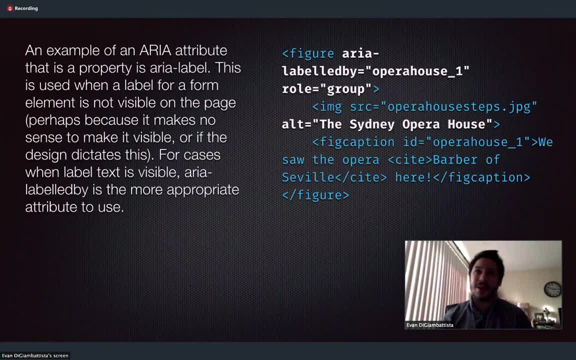 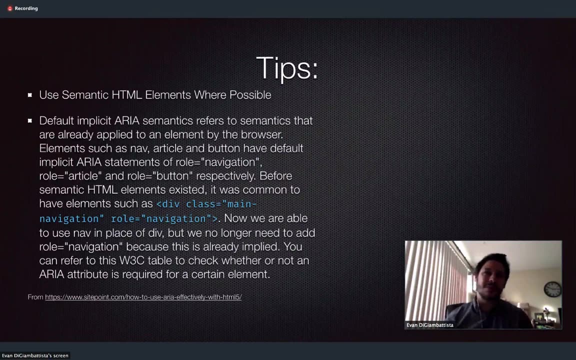 So off to the right in the code, example, ARIA, labeled by Opera House, underscore one role group That just sort of gives more information to a screen reader. Just in the interest of time, I'm just going to glaze through these tips.